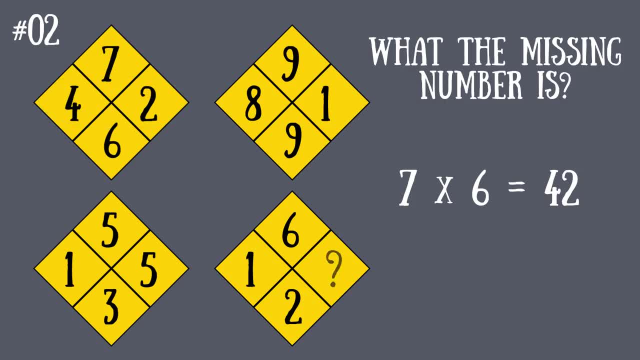 And that's exactly the numbers on the left and right. The same thing works for the other rhombuses. So in the last one, 6 multiplied by 2 is 12.. We already have number 1 on the left, which means the correct answer is 2.. 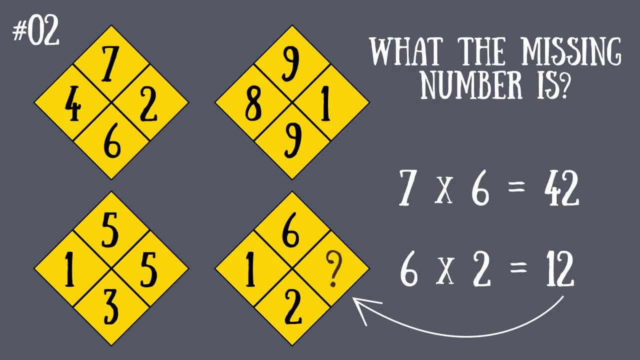 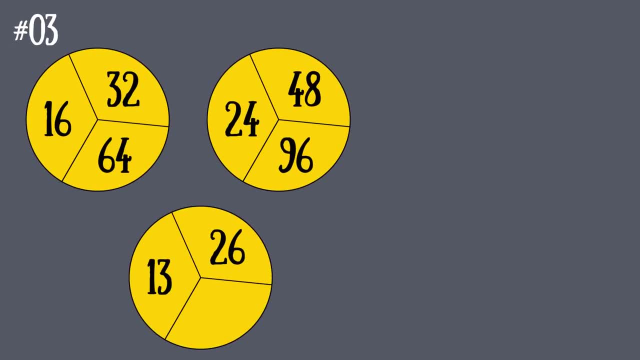 And I don't think I've said rhombuses so many times since about the eighth grade, Riddle number three: Here we have three circles, each divided into three parts, with numbers inside of them. Can you determine the pattern and figure out the number? 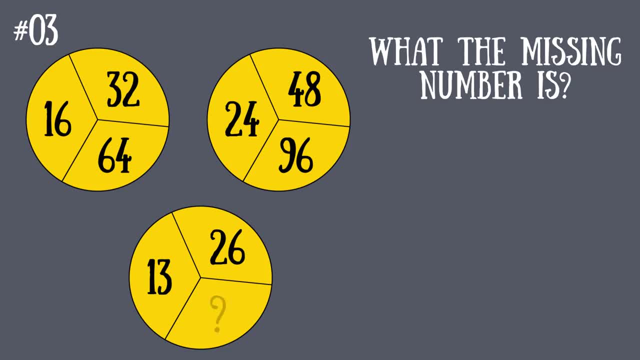 And figure out what the missing number is in the last circle. You have only 15 seconds, So do you have your answer ready? Look at the numbers closely. Let's start with the numbers on top, The number 32.. The number 32 is 16 multiplied by 2.. 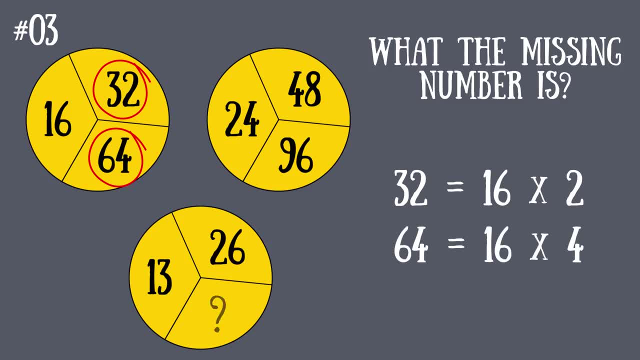 While 64 is 16 multiplied by 4.. Let's see whether it will work for the left parts: 24 multiplied by 2 is 48. And multiplied by 4 is 96. It works. So to find the missing number, we should just multiply 13 by 4, which is 52.. 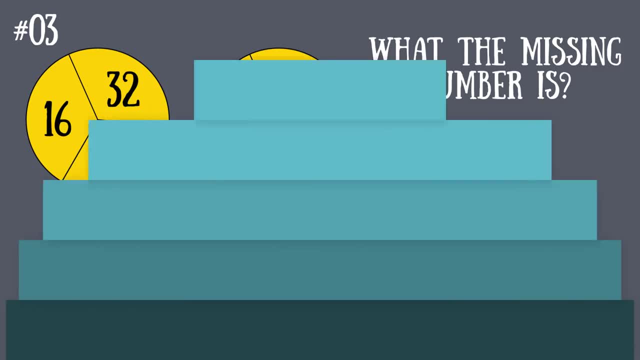 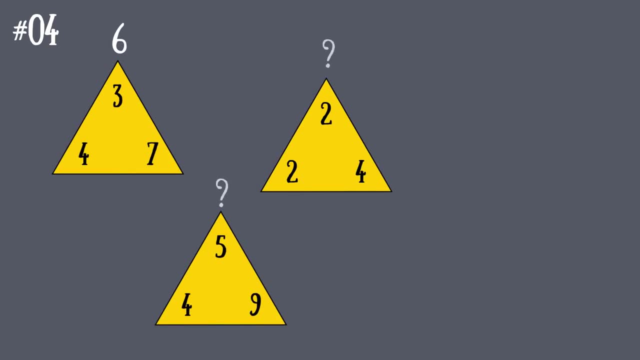 And that's the correct answer for you. Riddle number four: One triangle has all its numbers in place, But other two miss the numbers on top. Can you guess them? Try to find the correct pattern and use it in 15 seconds. 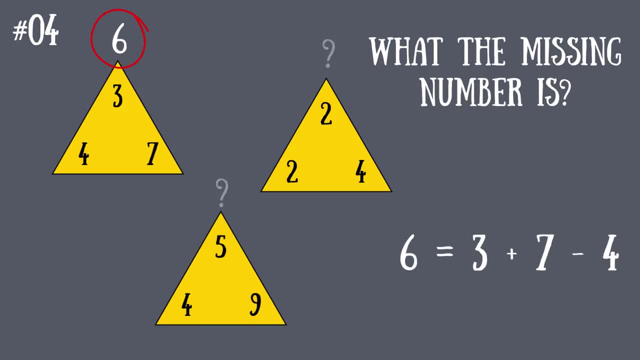 Let's start with the first triangle. Riddle number five. Let's start with the first triangle. How can we get 6? By adding 3 to 7 and subtracting 4.. And this is the exact correct pattern For the second triangle. it will be 4 plus 2 minus 2, which is 4.. 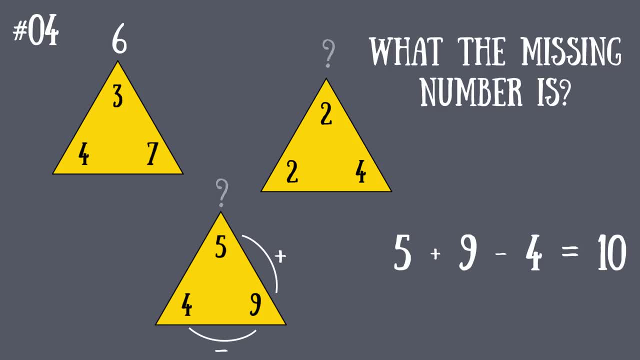 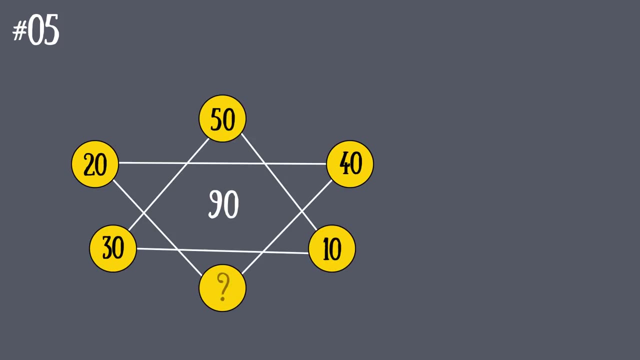 For the third one, 9 plus 5 minus 4 is 10.. So if you guessed 4 and 10, congratulations, you got it right. Riddle number five: Study the figure below. What number, in your opinion, is missing here? 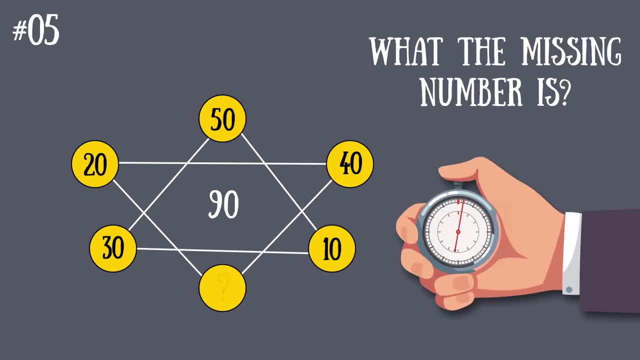 Time's a-tickin'. Well, the right answer is 30.. Look at the other triangle. There's a number 90 in the middle. If you sum all of its corners, you'll get it. 50 plus 30 plus 10 equals 90, right. 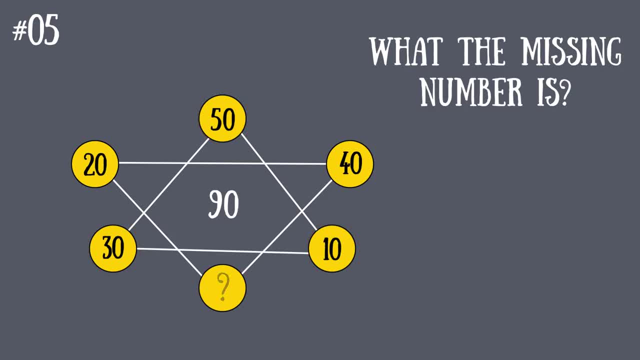 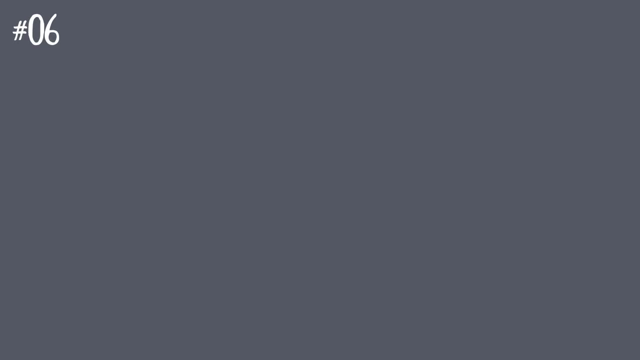 This same principle works for our triangle as well, because it also has 90 in the middle. So 90 minus 40 minus 20 is 30. Did you get it right? Tell us in the comments below. Riddle number six. 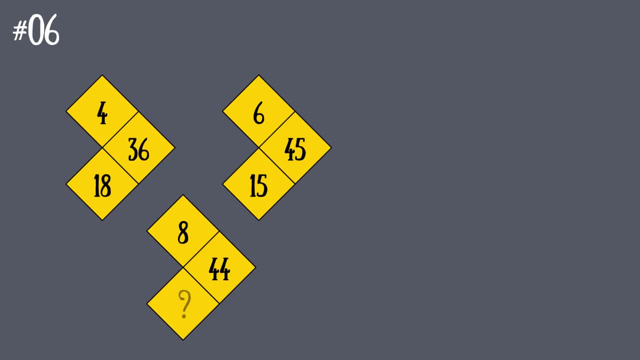 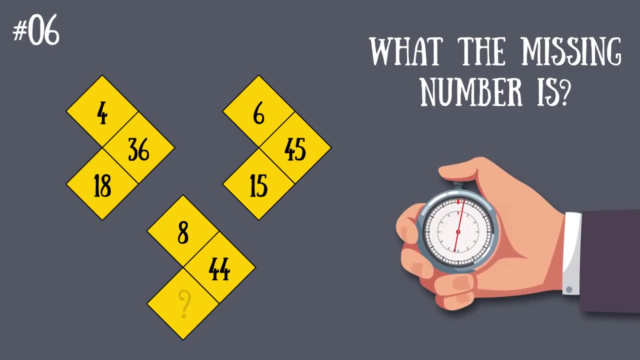 This is how your next task looks like. As you can see, one of the numbers in the bottom arrow is missing. You know what to do, Ready or not? it's time to find out the answer. The number on the right in each arrow. 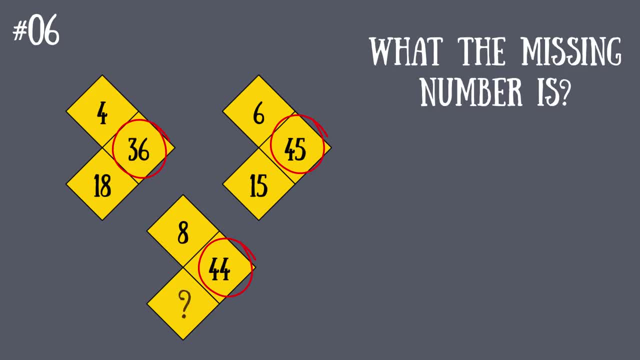 is the top number divided by 2, and multiplied by the bottom number. To make it a bit clearer in the first arrow, 4 divided by 2 is 2.. 2 multiplied by 18 is 36.. The pattern is found. 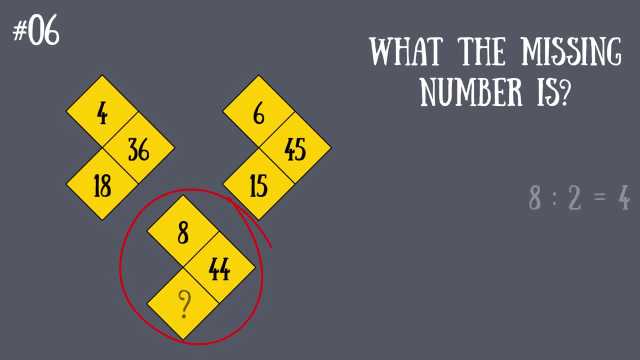 Now let's use it for the arrow we need: 8 divided by 2 is 4.. 44 divided by 4 is 11.. And that's it. The right number on the bottom arrow is 11.. Riddle number seven. 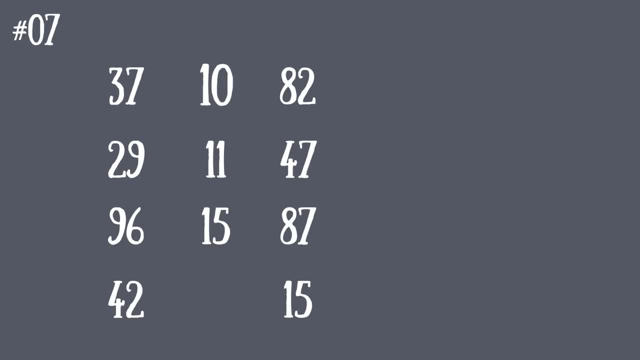 Four lines of numbers: 37,, 10,, 82,, 29,, 11,, 47,, 96,, 15,, 87,, 42, question mark 15.. So what number should be in the place of the question mark? 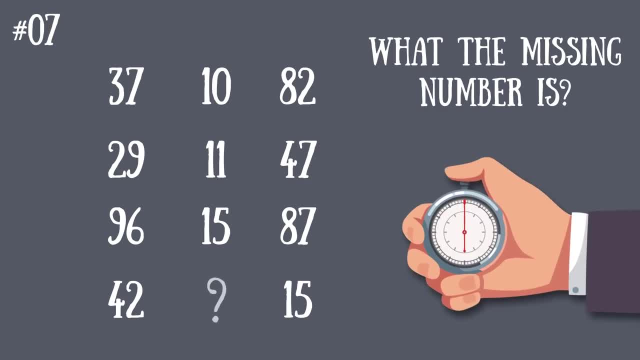 You have some time to think about it- 15 seconds, I think. Ready or not? here's an answer. The missing number is 6.. The number in the middle of each line is the same as the digits of either end's number added together. 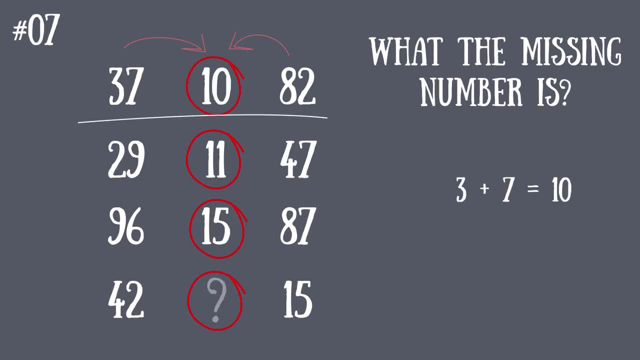 So for the first line, 3 plus 7 gives us 10, and 8 plus 2 equals 10 as well. That's why 10 is the number in the middle of each line. So let's apply the same principle for the last line. 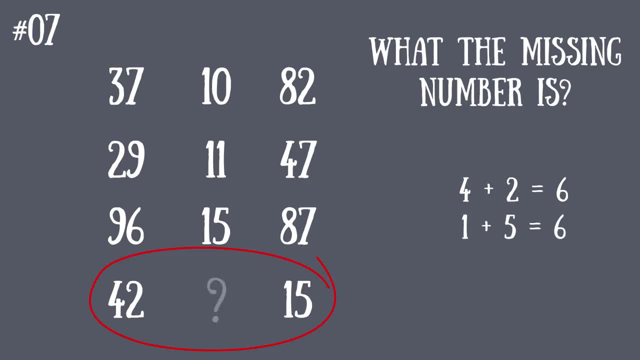 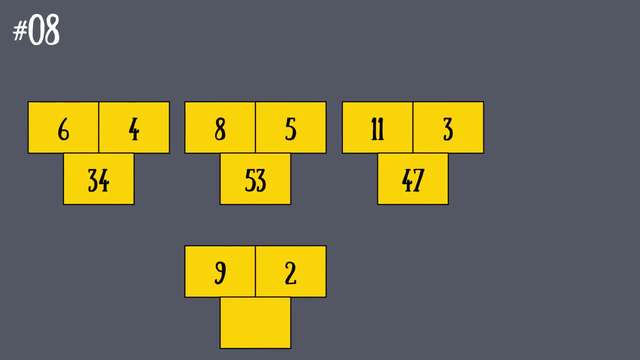 4 plus 2 is 6.. 1 plus 5 is also 6.. There you have it. Riddle number eight. The next puzzle is waiting for you. What number is missing here? Test your skills once again. So this is the correct pattern for this puzzle. 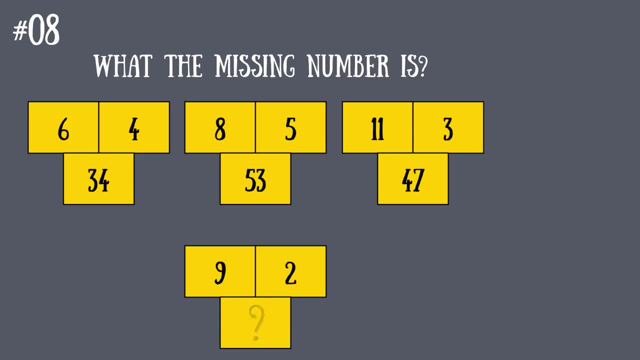 Check it with your numbers. The number at the bottom of each block is the sum of the top two numbers first multiplied and then added to one another. Simply, for the first block, it's 6 multiplied by 4, which is 24, plus 4 added to 6, which. 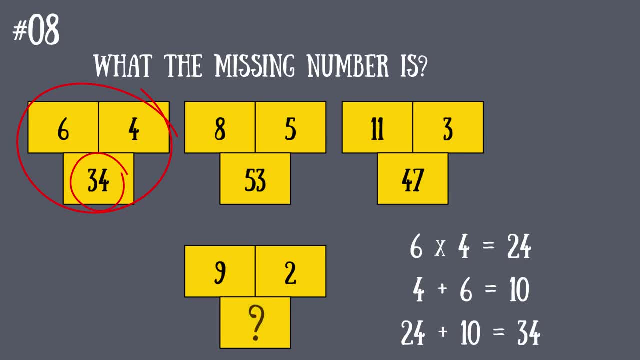 is 10.. 24 plus 10 equals 34.. Of course, this works for each block, so our number is 9 multiplied by 2, plus 2 added to 9.. That's 18 plus 11, which is 29.. 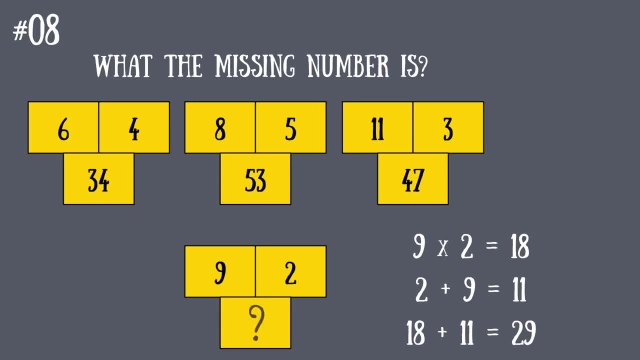 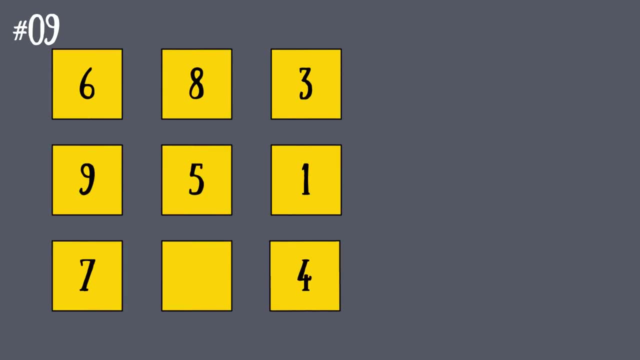 Props to you if you found this solution, but we're moving along to your next challenge, Riddle number nine, Another puzzle you have to solve. Look carefully at this picture, Sherlock. Your task is simple: Try to find the missing number in 15 seconds. 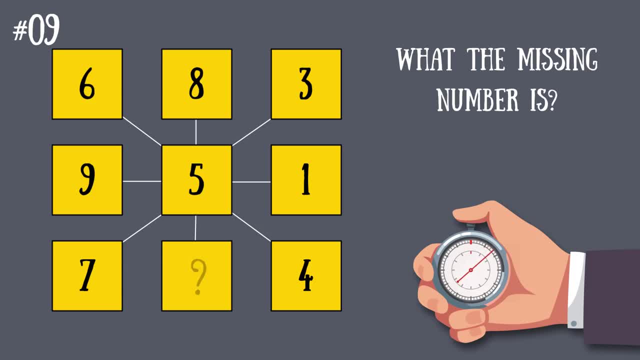 Well, I'm kinda lost, And you Well, here's the right pattern and answer for this mystery. If you sum the numbers of each line, you'll get 15.. For example, let's take the straight line in the middle. 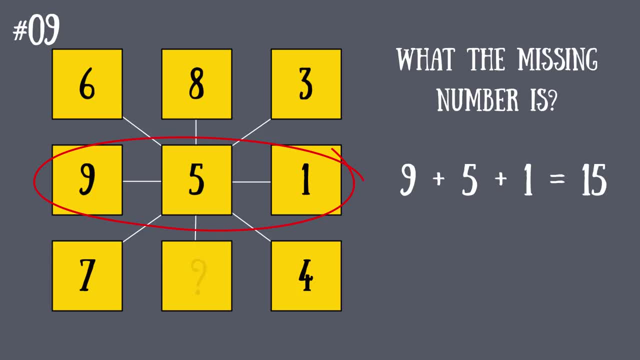 9 plus 5 plus 1 is 15,. right, This works for diagonal lines as well. The sum of 6,, 5, and 4 is 15.. 3,, 5, and 7 gives us 15 as well. 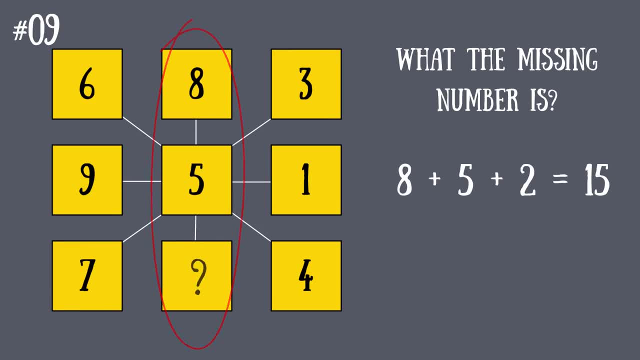 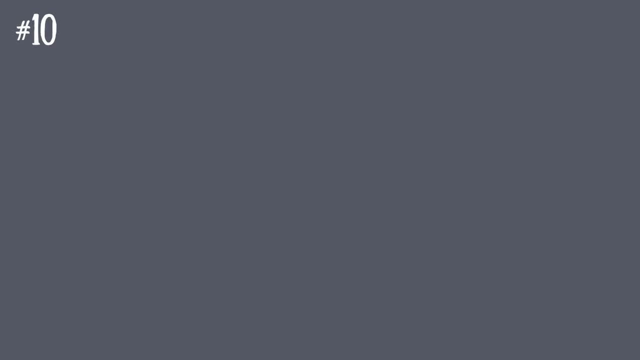 So the correct number here is 2.. 8 plus 5 plus 2 is 15.. Just what we need: 10. Riddle number 10. Riddle number 10.. 3,, 12,, 39,, 120, and…. 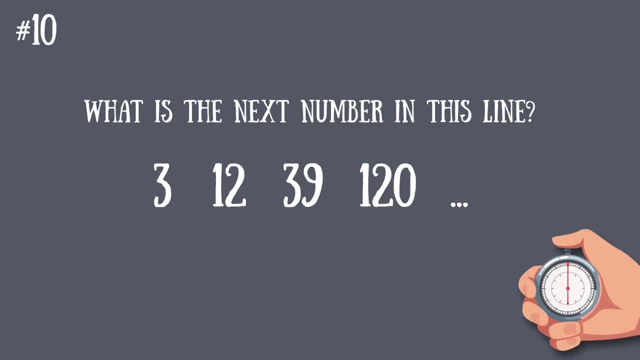 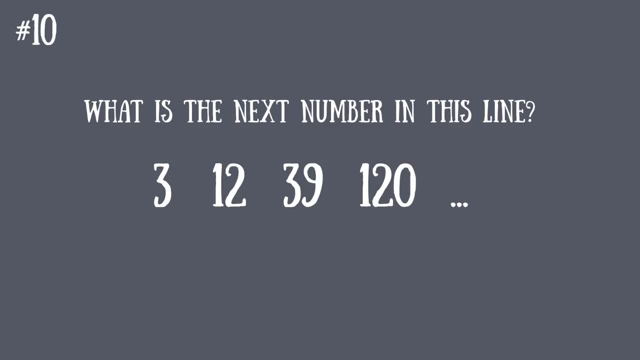 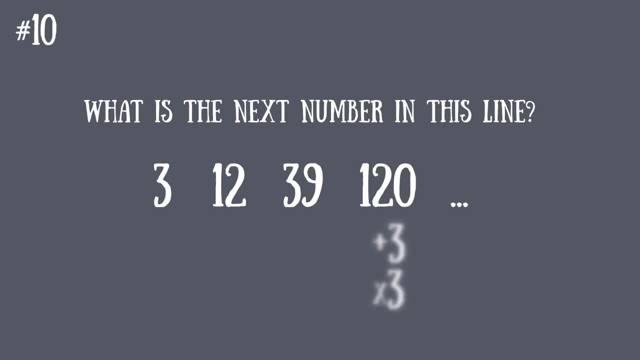 What will you do? What will you do? Err, You must have learned that you always have to figure out your acts in order to get done. The hidden secret is likely in the two gifts. 8 plus 11 are for children. I'll find it out about them when we get them out, okay. 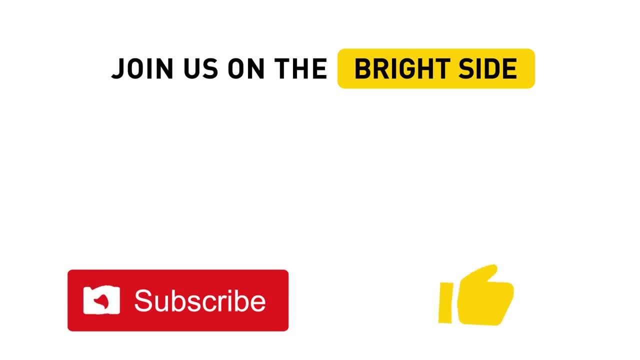 It definitely needs to be about them in the hospital. We'll come back with you with another level to figure out how to solve your riddles in an easy way. Kir, HAVE a good day. Don't forget to hit the like button, share this video with your friends and subscribe. 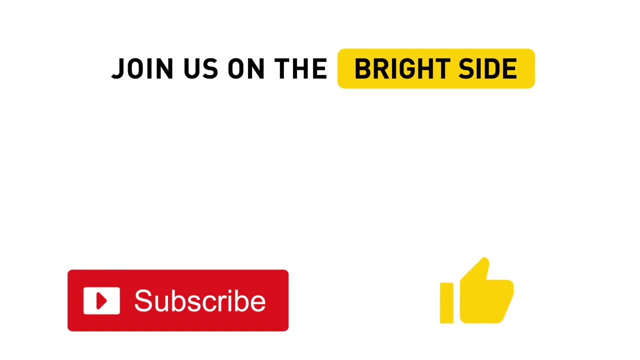 to our channel if you want to stay on the Bright Side of life with us. See you soon.